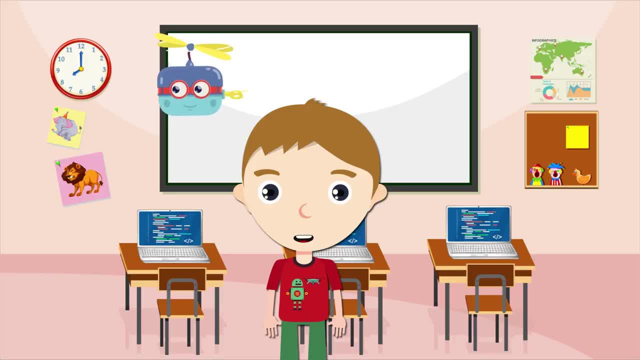 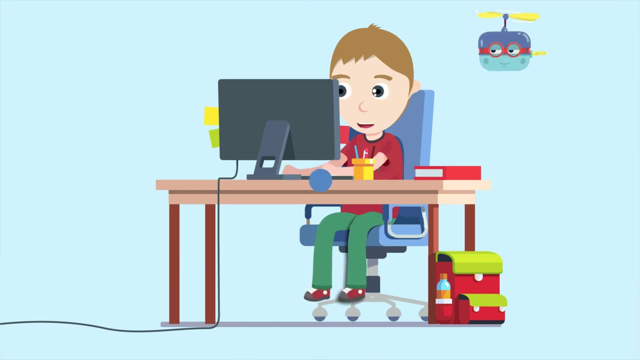 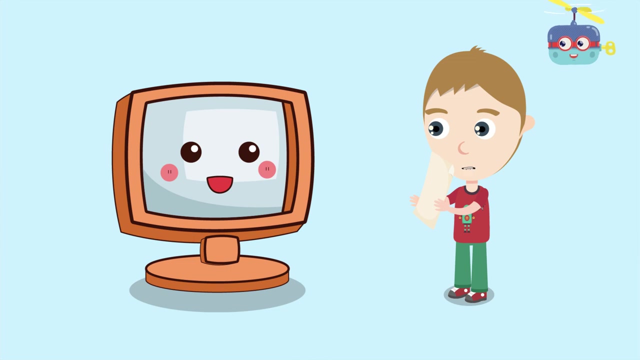 Number one: Algorithm. An algorithm is an instruction given in order to complete a certain task and receive the desired result. So a computer programmer will write an algorithm to tell the computer how to perform a certain task to produce a result. It's just like getting dressed. 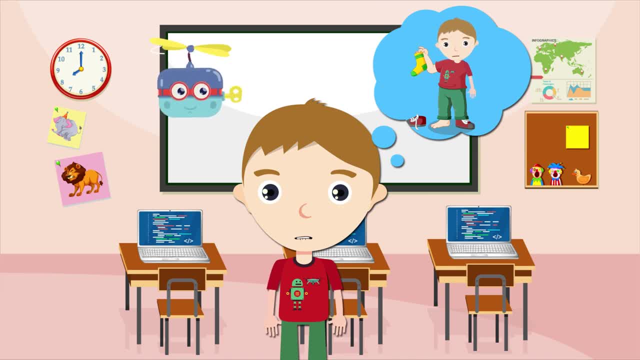 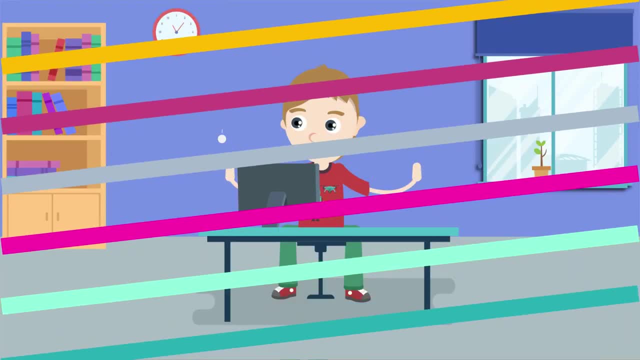 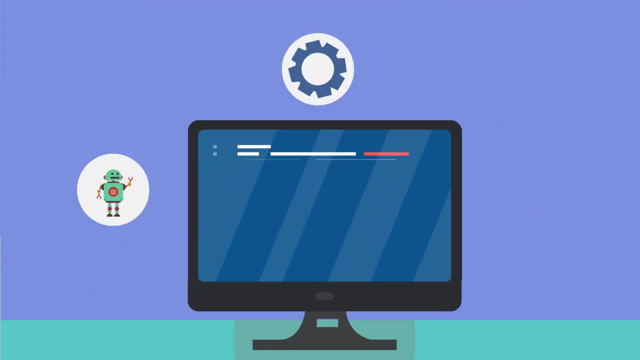 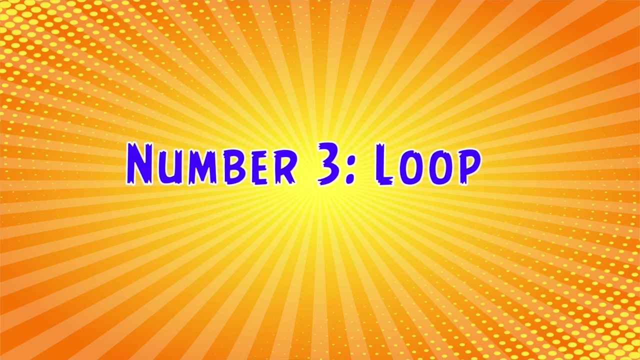 You can't put your shoes on Before your socks. Number two: Sequence. Sequence is basically completing a task in a certain order. So if we think about algorithms, it means putting those instructions in order. Number three: Loop. Something that goes round and round again and again. Right, 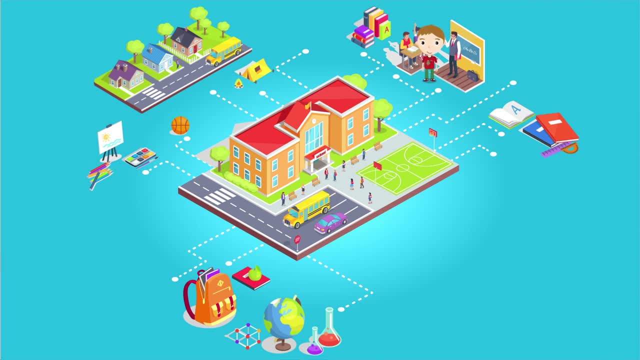 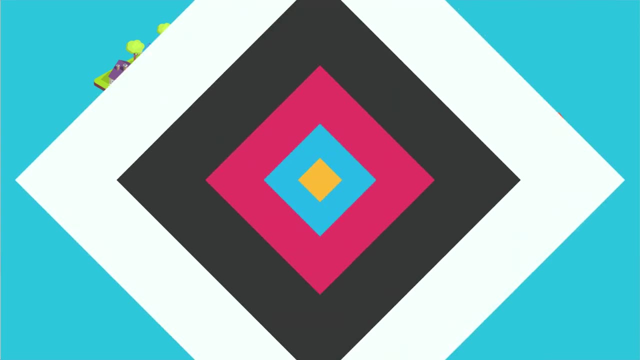 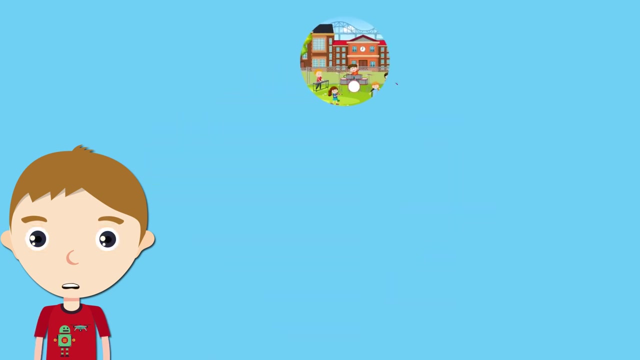 Think about the steps you would need to follow to travel to school every day. This is a good example of a loop. Wouldn't it be a lot simpler if we don't have to repeat all these steps every time we went to school? Since every day we repeat the same steps, this is considered as a loop. 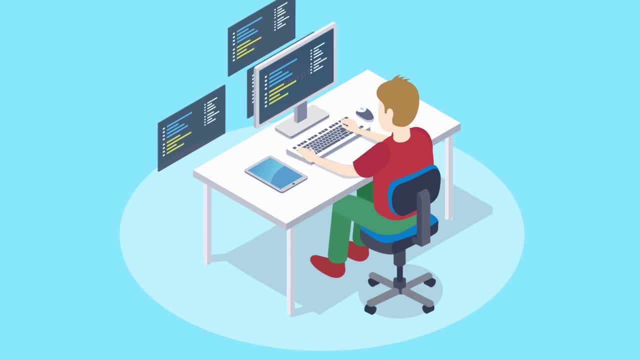 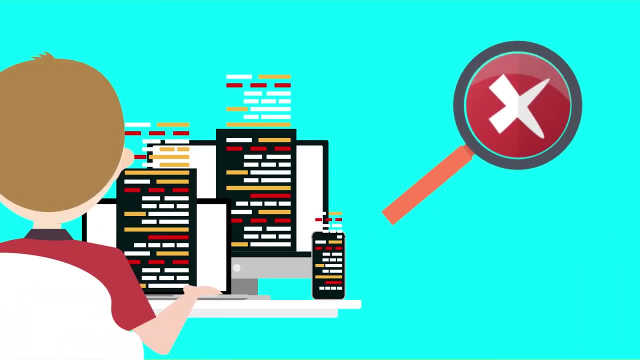 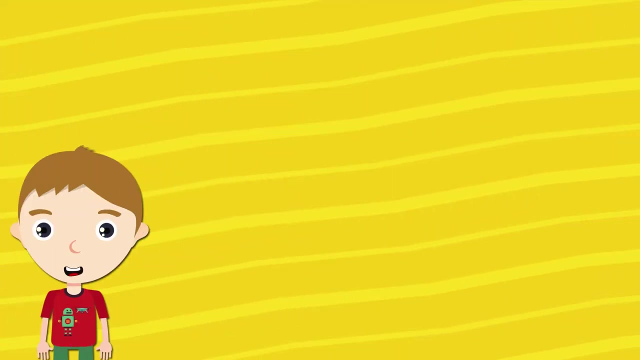 Computer programmers use loops to make their programs work. They use loops to make their programs more efficient. Number four: Branch. Branching basically means checking conditions which determine the choice being made. So in other words, making a decision depending on what is happening or what has happened. 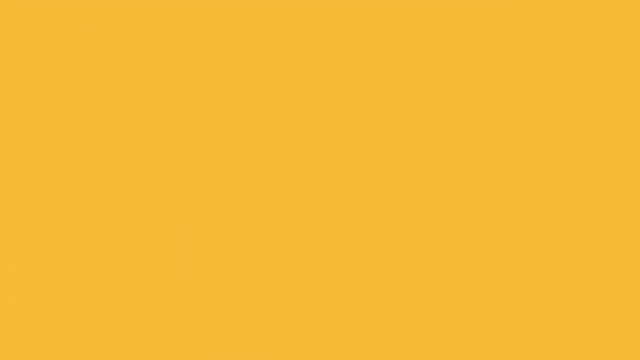 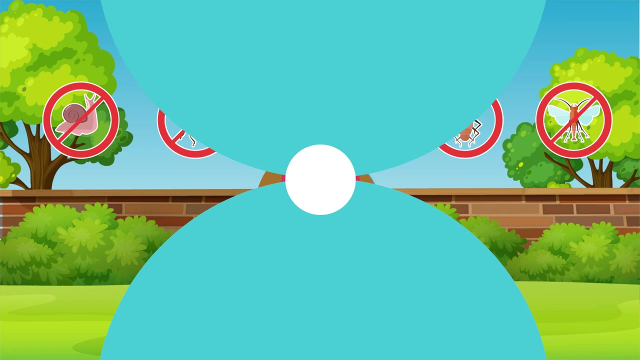 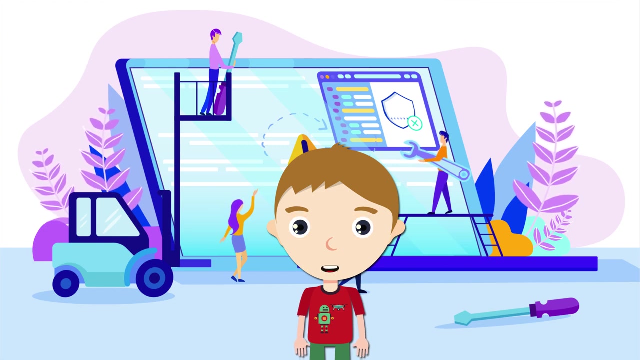 Number five: Debug. Debugging has nothing to do with programming. Debugging has nothing to do with bugs and insects that you find in the garden. Debugging is basically fixing an issue that you come across within instructions in order to produce your desired result. 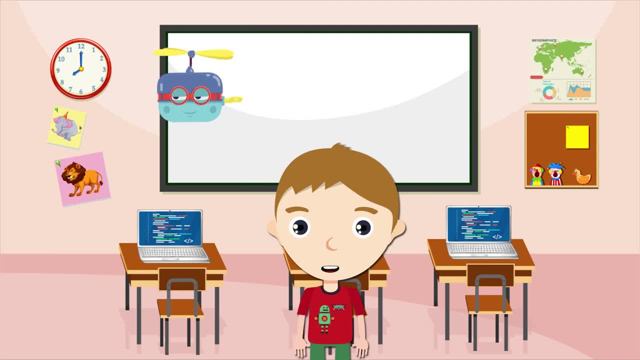 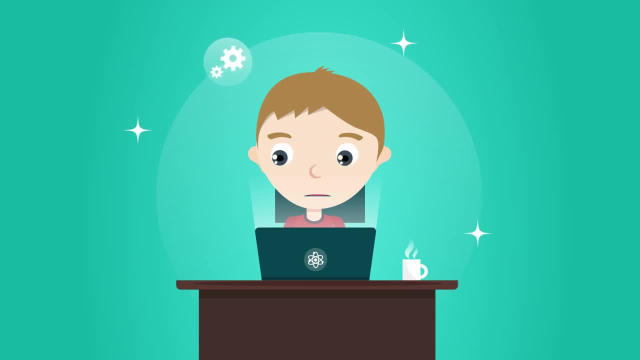 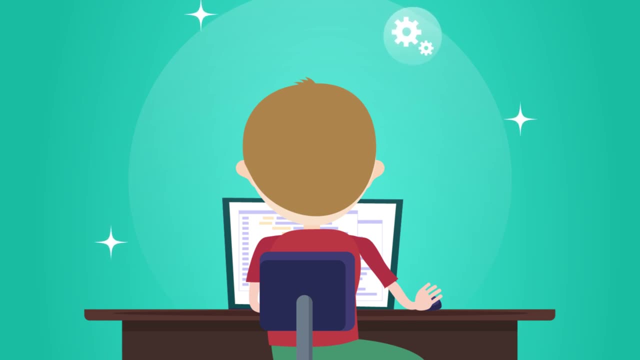 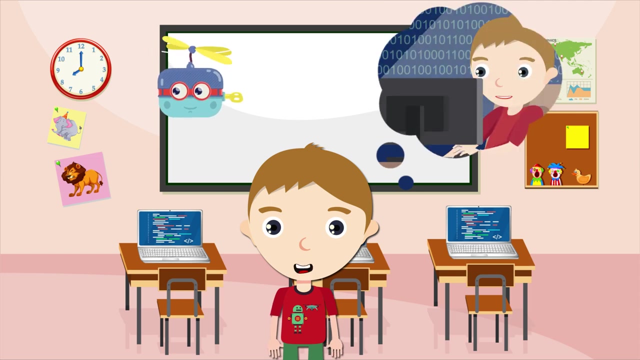 Debugging isn't always the easiest coding concept to understand. You may become impatient, You may want the answer right there, and then It is an important coding concept to learn because problem solving plays a large part in computer programming. Well, I'm off to do some coding. See you soon.